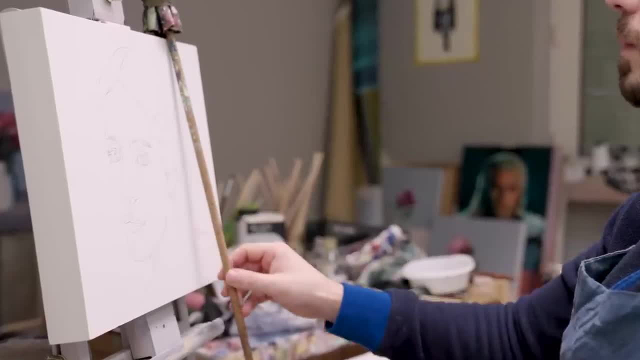 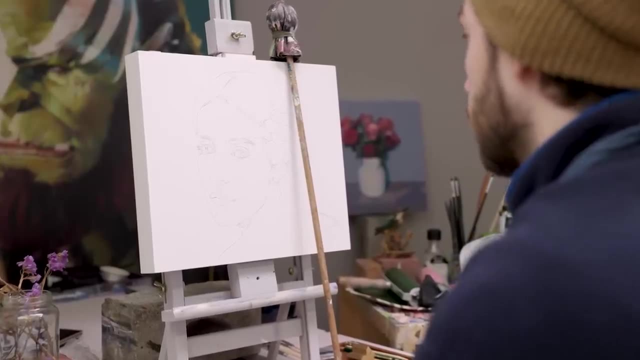 paintings that many of you have been asking me to paint for quite some time. So buckle up and let's find out how anything can be painted in just four simple steps. And if you want to dive even deeper into the process of how I painted this beautiful young lady here, make sure to head over. 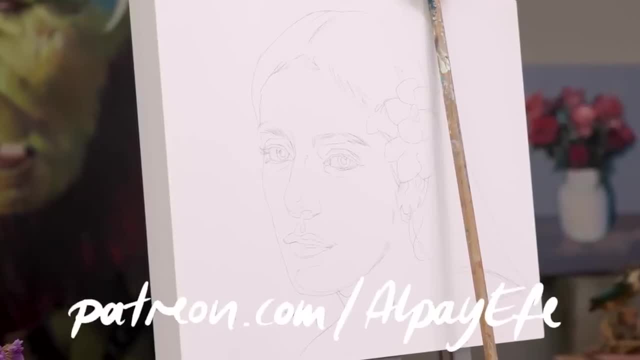 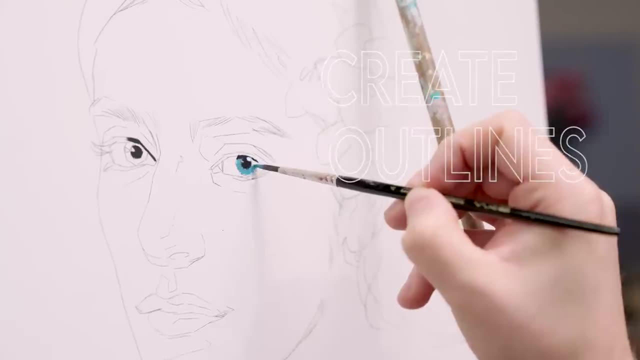 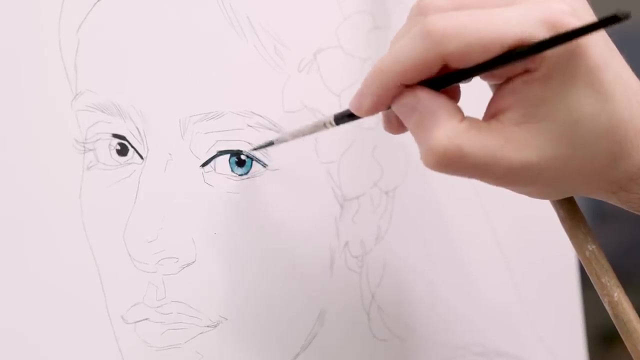 to Patreon, where you can find an extended version for this and many of my other videos. Step 1. Create outlines. Every artist has experienced this at some point. For example, you're painting a face, focusing on mixing colors and being super accurate, capturing. 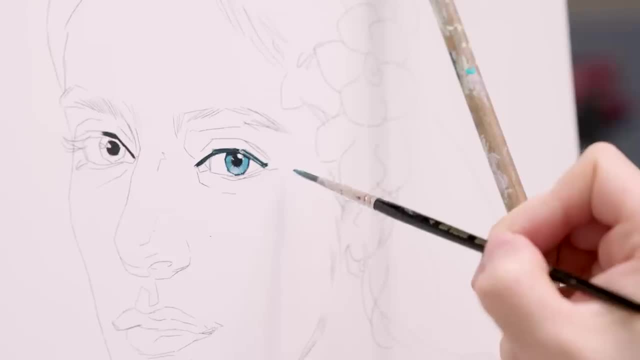 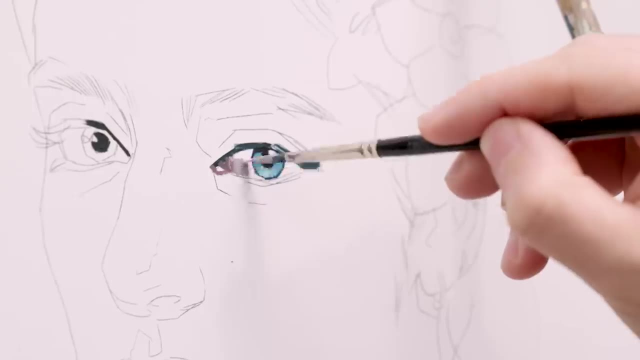 every detail. But when you finally take a step back, after many, many hours of focused hard work, you realize that there's a lot of work to be done. You start to see that you're work. you realize that somehow, somewhere along the way, things have gone sideways. 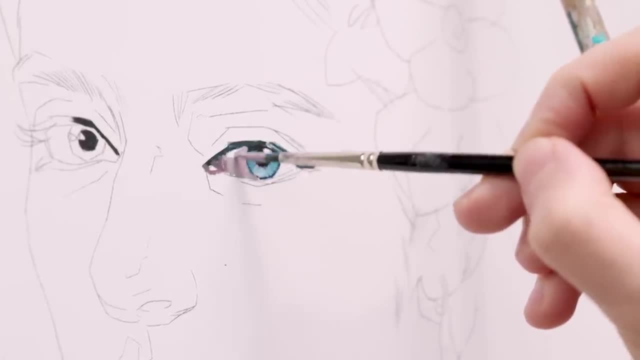 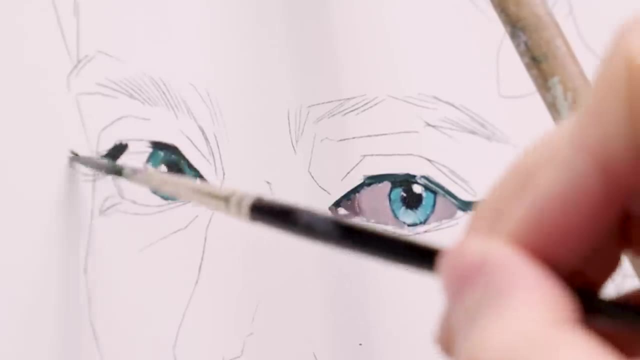 The forehead is big enough to project a movie onto it, the lips are thin and don't have any volume and, for whatever reason, you have managed to somehow paint a face from three different perspectives at the same time. But the eyes you've painted look pretty decent, if only one of them wasn't three. 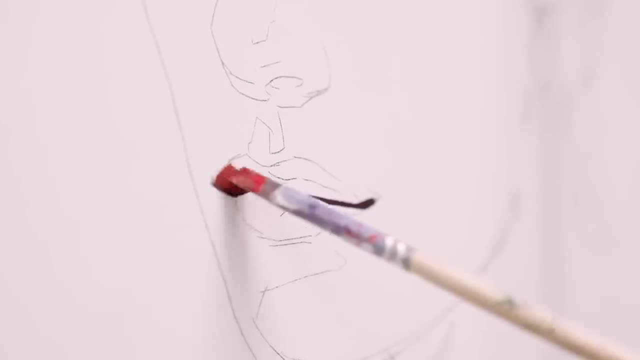 times as big as the other one. This is precisely why we start our paintings with an accurate drawing, or, how I like to call it, outlines. Painting itself is already hard enough: mixing colors, creating the illusion of light and shadow, painting transitions, creating texture. 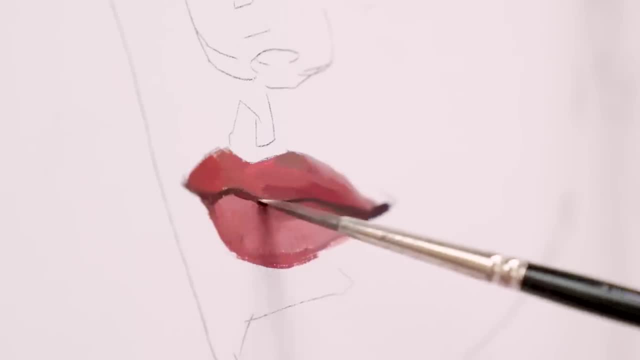 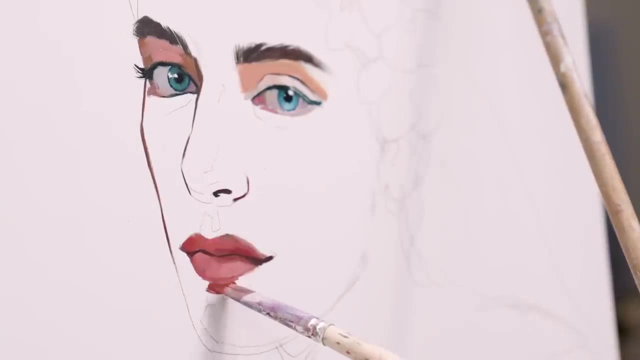 But doing all of that while trying to get proportions, anatomy or compositions right is, more often than not, a complete nightmare, especially for people who don't have years and years of practice and experience. This is why the first step in painting anything is to take this part out of the equation and 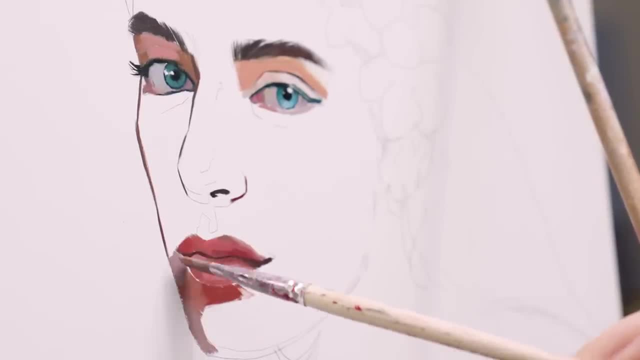 to deal with it before you even put down your first brushstroke. Doing this allows you to focus on a few things. For example, if you want to paint a painting, you can start with a brush stroke. You can start with a brush stroke. 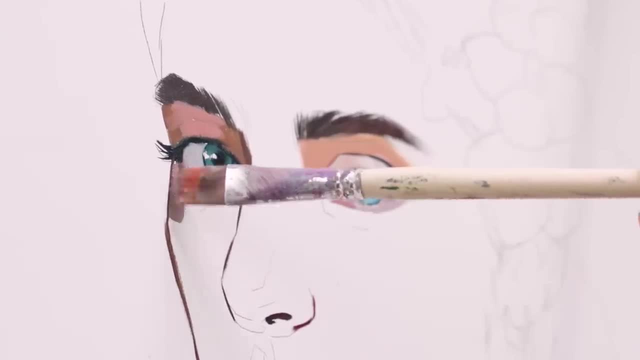 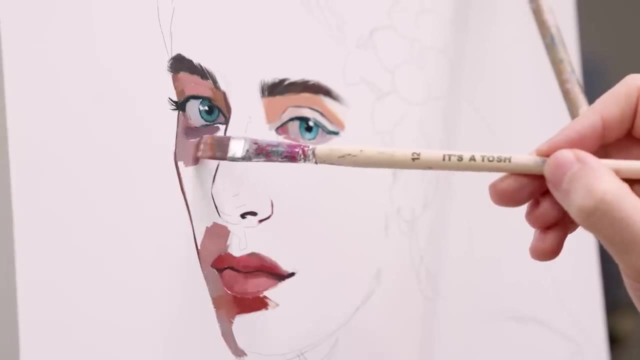 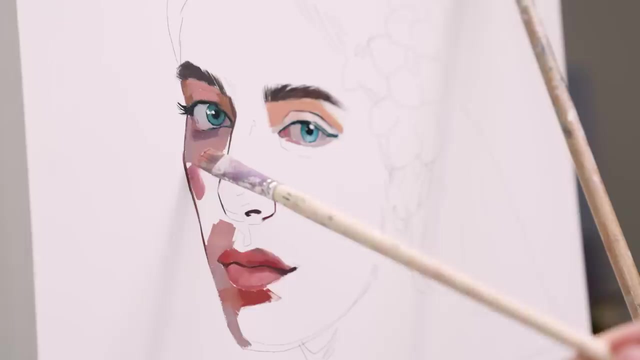 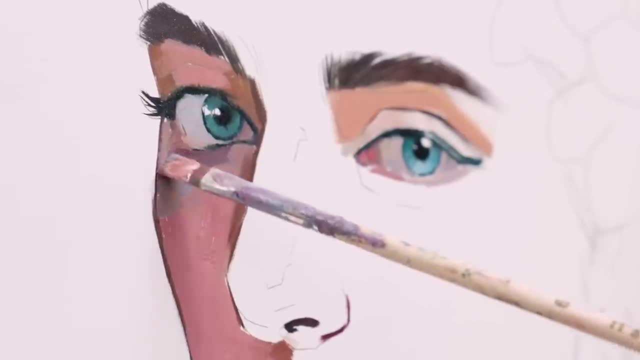 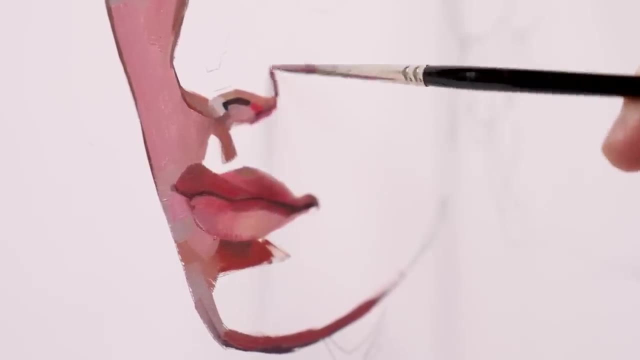 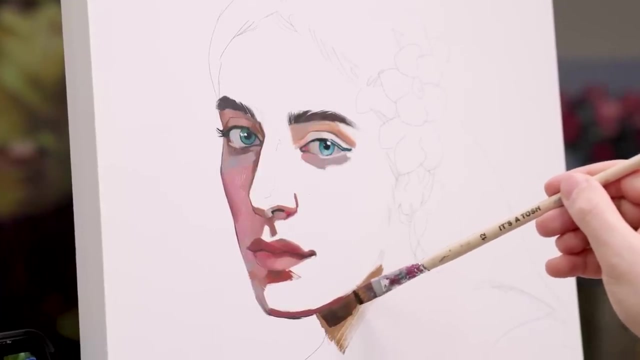 or what they call it. whatever surface and then start painting. In my opinion, not the best approach for various reasons. Others use a form of grid method to translate their reference to their painting surface. Especially when you get to bigger paintings, this is almost inevitable. You can use a projector or a transfer method, or 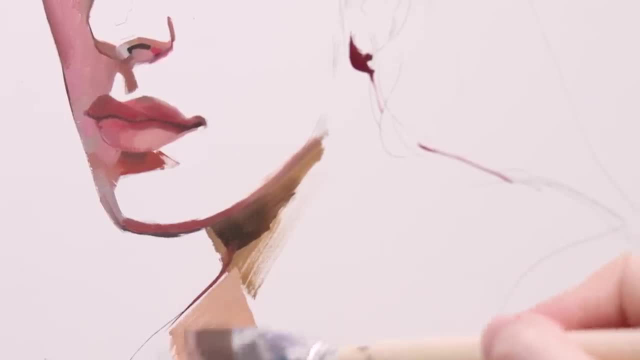 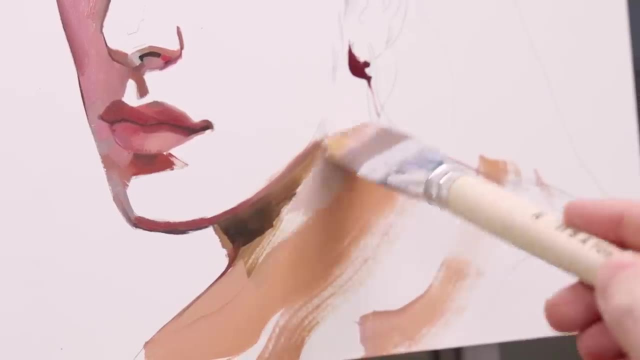 you can use a combination of the above, For example, creating a drawing and then transferring or projecting that drawing onto your canvas. Each method has its advantages and disadvantages, but they all give you the same result. I personally prefer to use something like a projector most of. 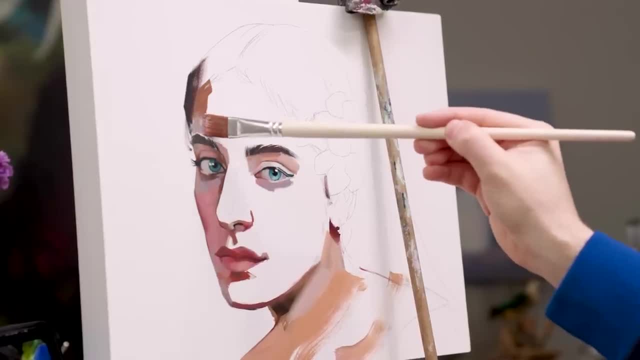 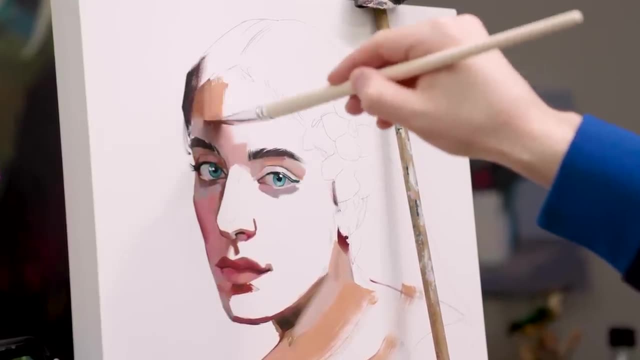 the time because, honestly, I can't be bothered with spending hours and hours on what's essentially just prep work. for me As a professional artist, my focus is to constantly produce the best work that I can, as effectively and efficiently as possible, and skipping the drawing part altogether. 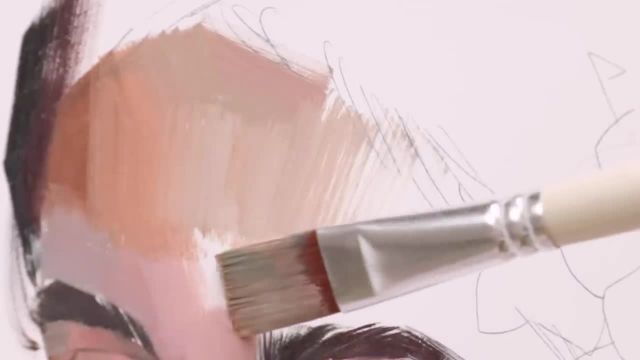 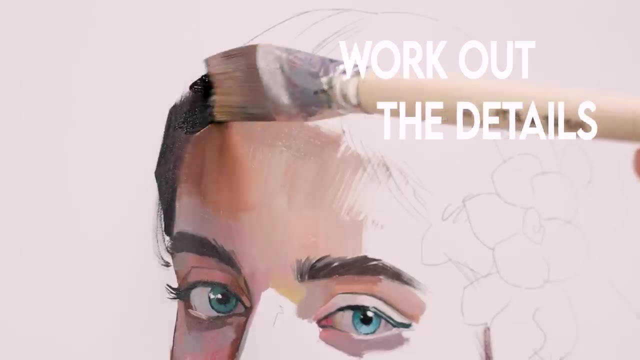 not only lets me do this best, but it also suits my painting style the best, But your mileage, of course, may vary. Step two: Work out the details. The next step is to create a project that you can use for your work. The next step might sound counterintuitive, especially for people familiar with traditional 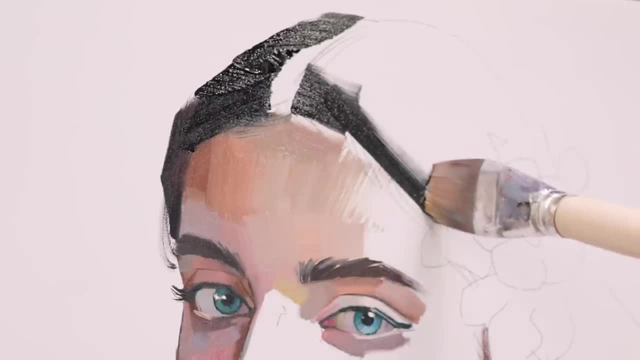 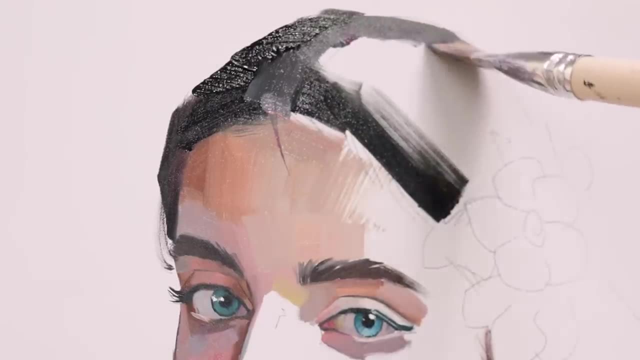 drawing or painting bits of advice, but in my experience it helps most people draw and paint anything they want in a simple and straightforward way, and it's to start with the most complex and detailed areas of what you're painting first. One of the most common art advice that you will. 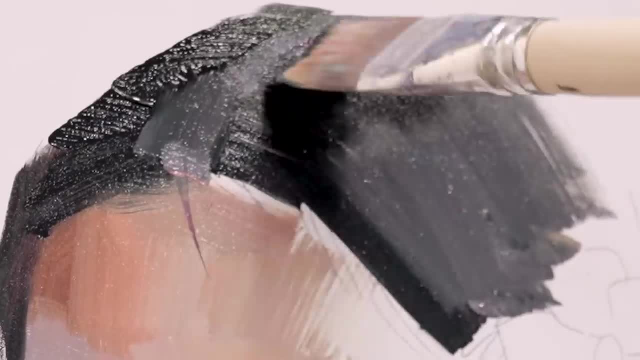 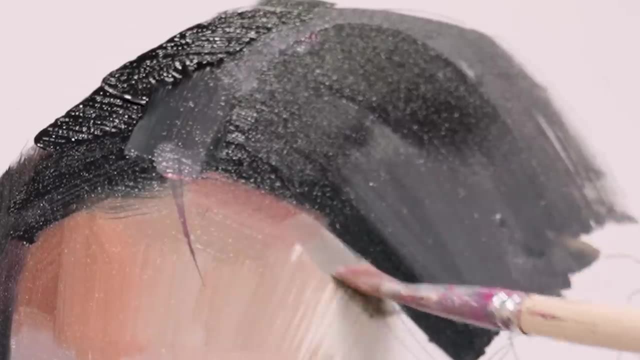 come across is to start with big shapes, Start your painting very rough or loose and then gradually get more detailed and refined. This isn't necessarily bad advice, because if you have the skills and the knowledge to pull this way of painting off, it is one of the most. 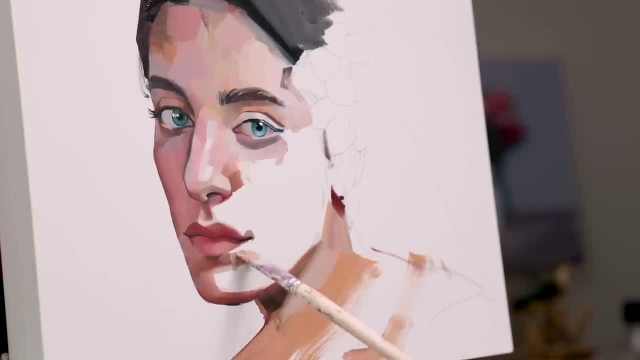 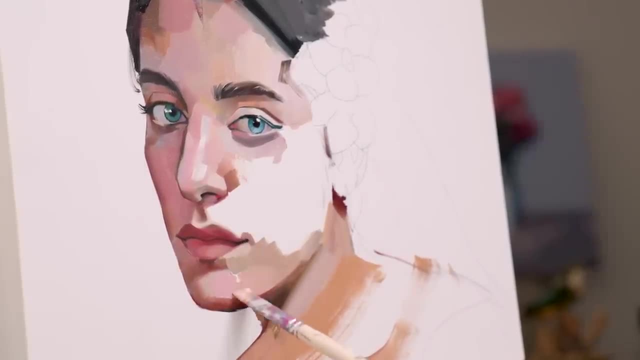 visually pleasing and impressive, but if you don't- and believe me, most people don't- it's probably not going to work for you. Starting with big shapes and getting more refined is pretty much painting, drawing and figuring out proportions at the same time. It's already hard to do just one of these. 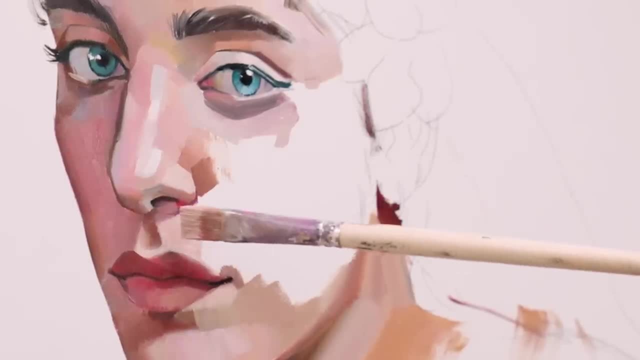 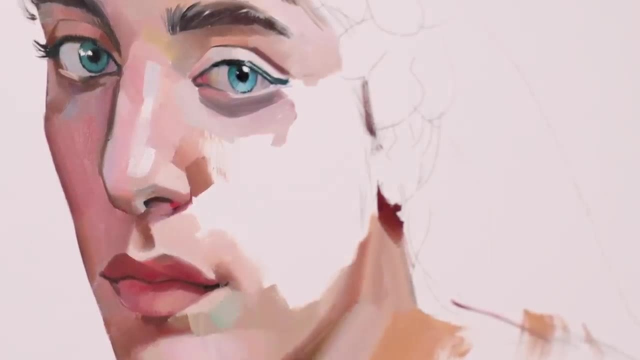 things, let alone do all of these things simultaneously. From a technical and psychological point of view, it makes a lot of sense to focus on the complicated stuff, But if you're not sure what you're painting, it's tough first and then to move on to other things A painting can take. 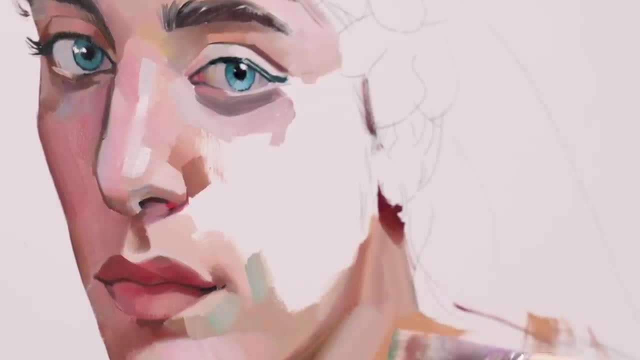 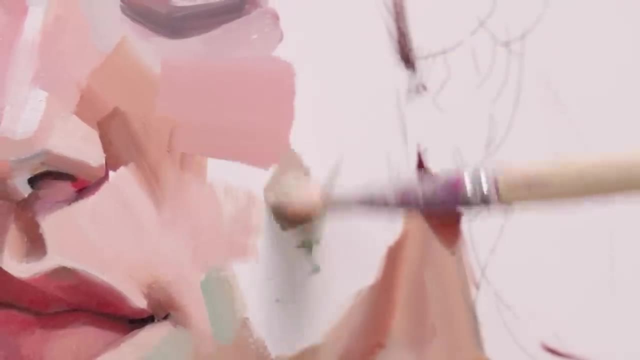 anywhere from a few hours to a few days or even weeks. It makes sense to use the initial burst of energy and enthusiasm that you typically have at the beginning of a project to get some of the most challenging and most important parts out of the way. It's rewarding and motivating, and it 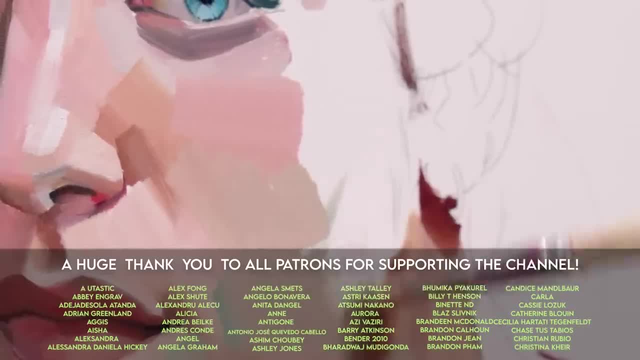 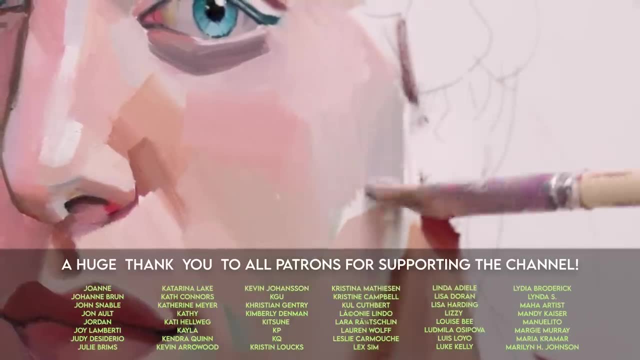 encourages you to keep going because things are already looking promising. But also from a technical point of view, this makes sense. I started this painting, for example, by painting the eyes first, Arguably the most essential element of the image, Focusing on this part first before doing anything. 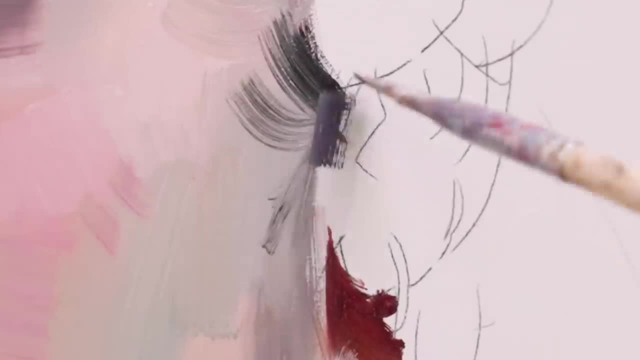 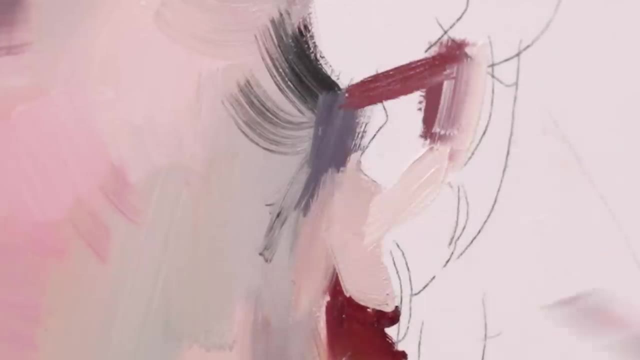 else makes sure that I get this absolutely fundamental part right from the very beginning. There is nothing more frustrating and demotivating than running into problems halfway through a project. You're going to run into problems all the time anyway, but the complicated stuff is really. 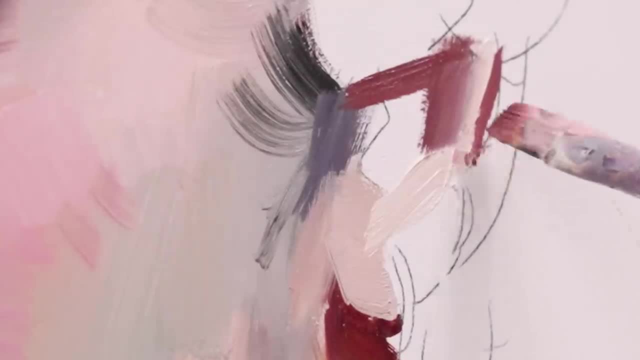 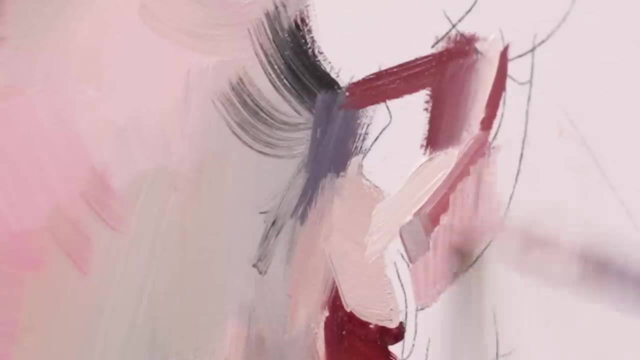 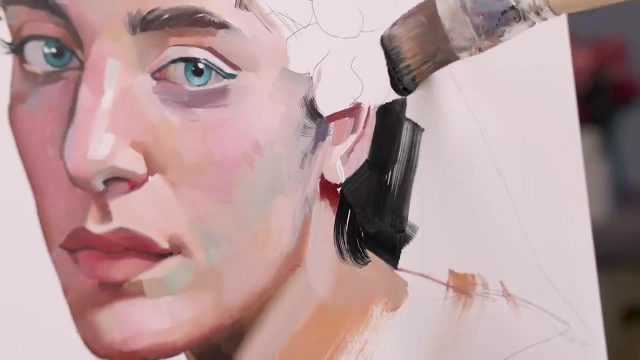 hard to fix. Fixing a composition- Absolute nightmare. Moving an eye one centimeter to the left. If you've ever tried that, you know that you might as well start a completely new painting at that point instead of bothering. And the same goes for lips or the nose. But fixing something like a hairline or 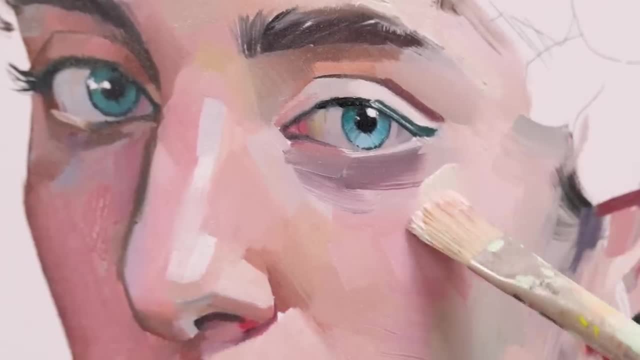 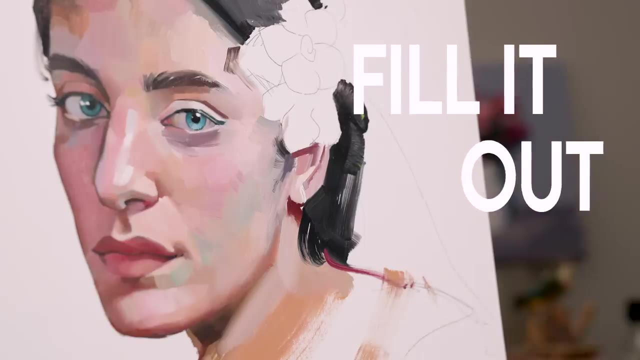 color is relatively easy. So start with the complex stuff first. get it right from the start and then enjoy a smooth ride. Step 3. Fill it out With all the complex stuff out of the way. we can finally relax a bit. This is the part where you 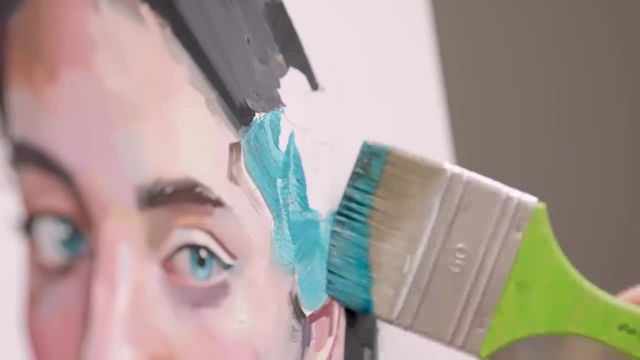 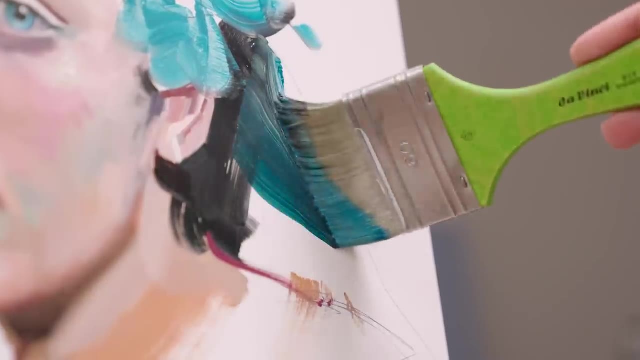 can actually be a bit looser and ease up a bit. The main goal of this step is to get paint onto the painting surface and to finally cover it up. This step is less about accuracy and more about creating the overall look for the whole painting. Color, harmony, brushwork, texture With this. 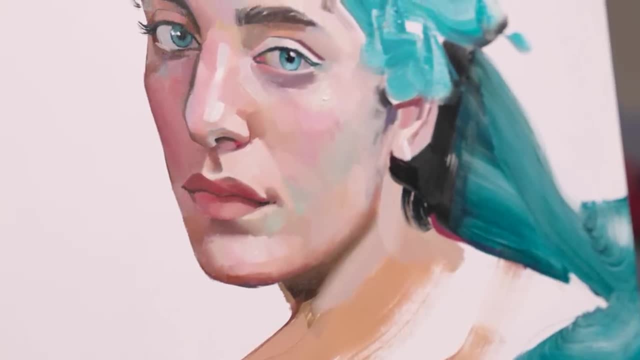 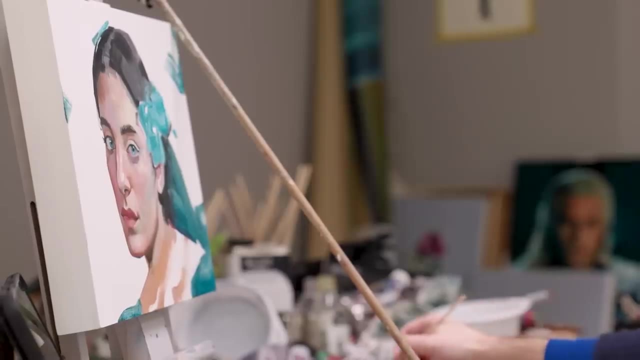 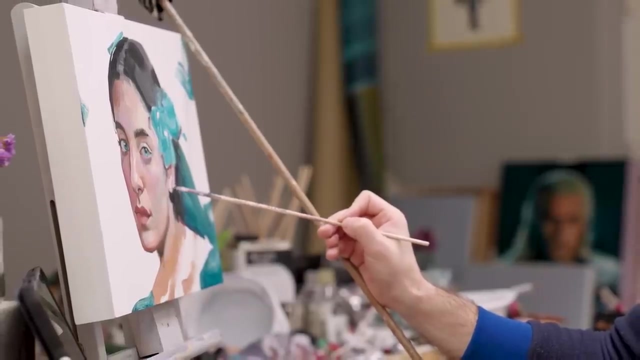 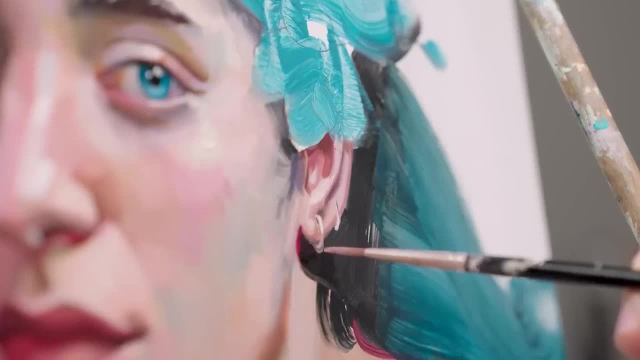 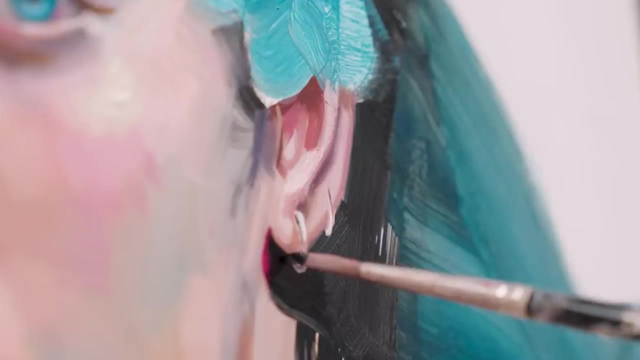 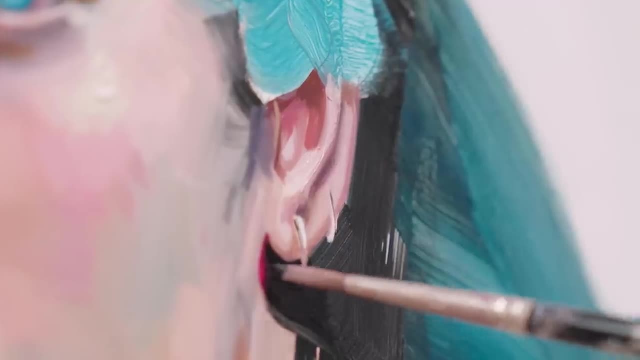 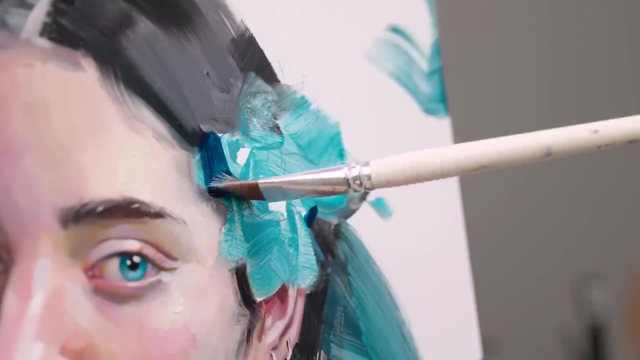 going to have to come back and tweak things. anyway. You can really go as simple or as complicated as you want here. You can just put patches of color next to each other until your painting looks loose yet close to finished, Or you can spend more time on rendering individual areas. 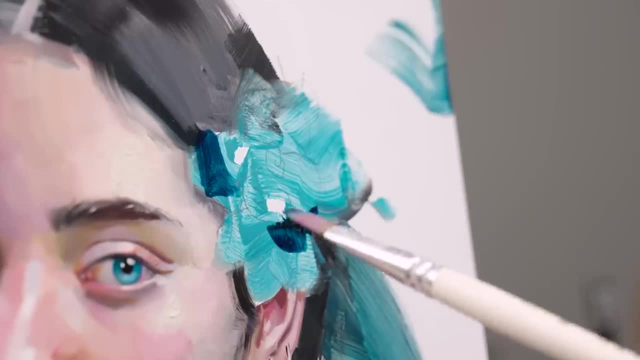 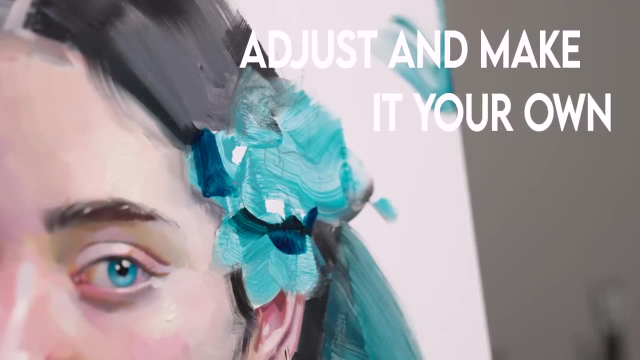 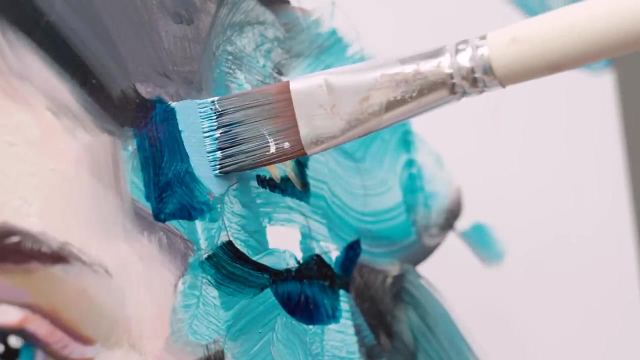 of the painting to make them stand out. Either way, the goal is to fill everything out before moving on to the last step. Step four: Adjust and make it your own. In the end, there will always be areas or parts of a painting that will need some adjustments, Areas that are too light or dark. 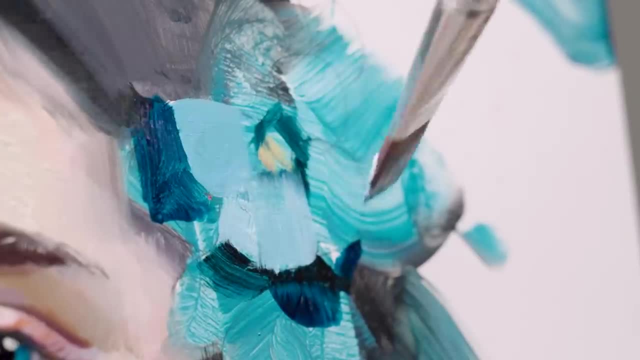 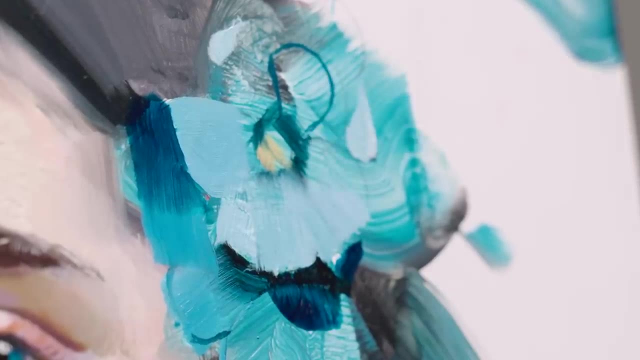 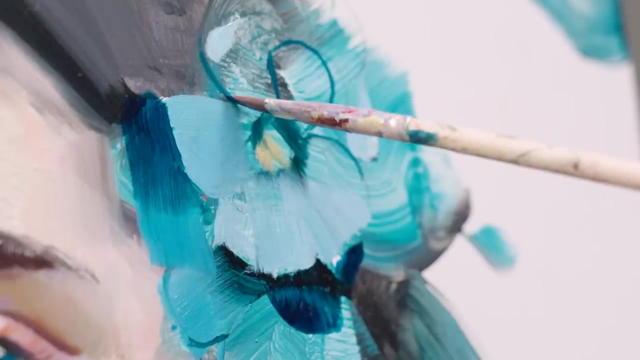 Areas that are too busy or proportions that aren't 100% right. This is the part where you can fix all of those issues, But this is also the part where you can make a painting your own. Whatever it is you've painted, you probably didn't manage to 100% capture or replicate it at this point, So if you 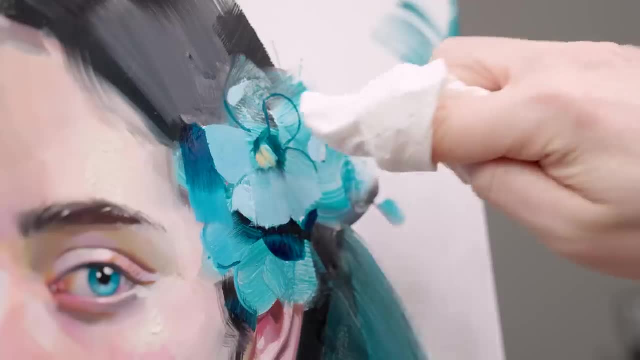 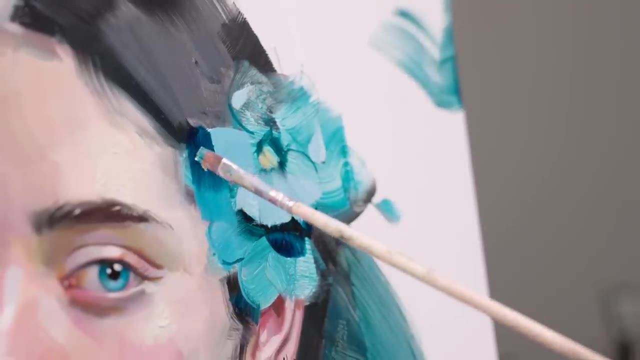 ask me- and this is just my personal opinion- you might as well add or change things to your own liking to make it your own. This step is arguably one of the most important, but also, unfortunately, one of the most underappreciated. Believe it or not, you are free to change colors, add things or 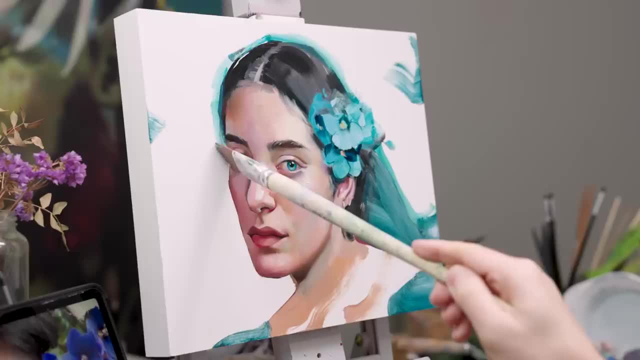 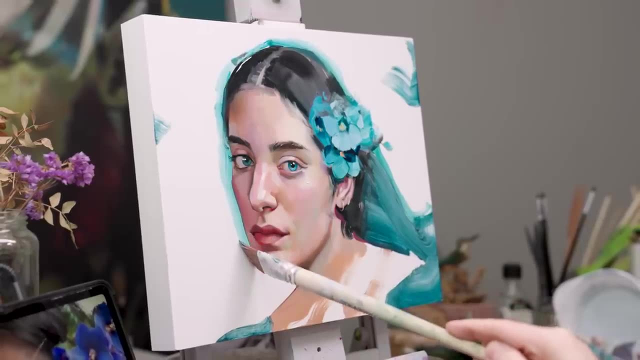 take stuff away according to your own liking. You don't have to just paint something the way you see it. I've said it before and I'll happily say it again: Painting what you see will also only get you what you see, And nine times out of ten, if you are painting something from real life, it's going to be. 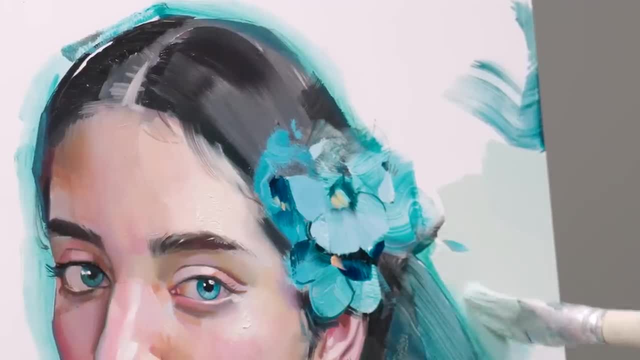 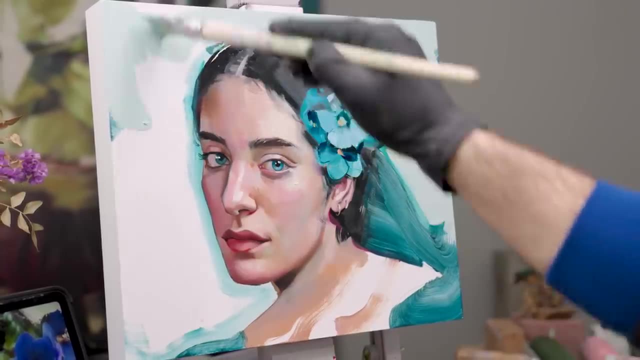 boring as hell. I personally like to paint more intuitively. at this point, and more often than not, I will completely put my reference aside and just focus on my own painting. In the case of this painting, this means to use color and techniques like design elements. Hair turns into brush strokes. 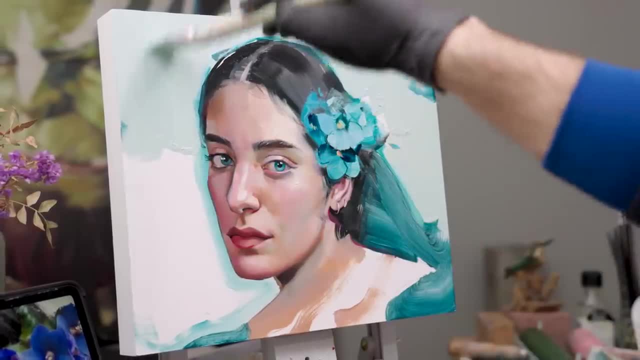